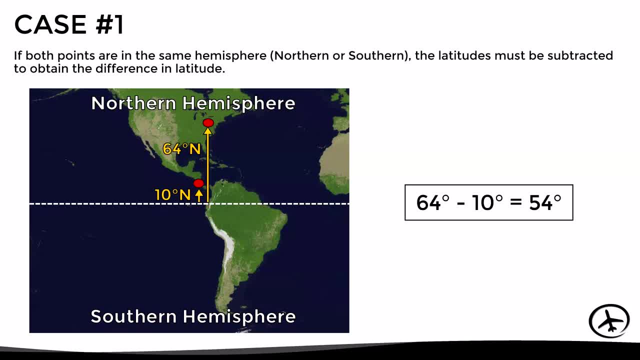 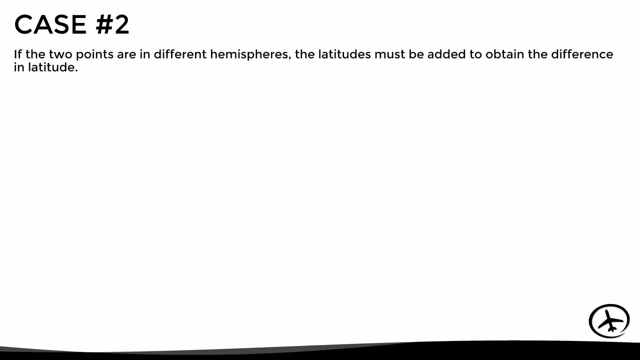 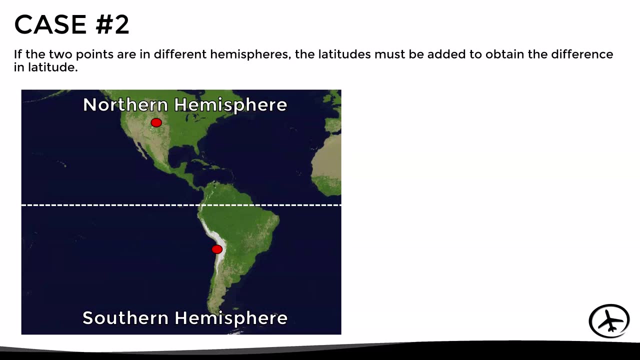 hemisphere, so we subtract the latitudes and obtain a difference in latitude of 54 degrees. On the other hand, if the two points are in different hemispheres, then the latitudes must be added to obtain the difference in latitude. In this example, one point is in the northern hemisphere while the other is in the southern. 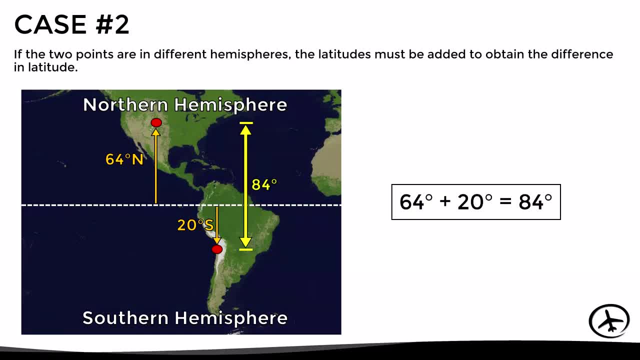 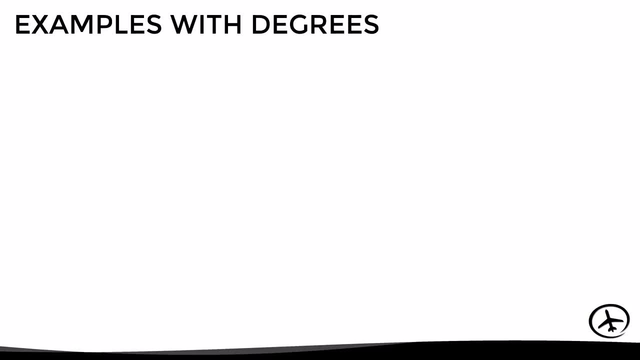 hemisphere. so we add the latitudes and obtain a difference in latitude of 84 degrees. With this being said, let's look at some examples. In this first case, we can see that both points are in the northern hemisphere. so we just subtract the latitudes and obtain a difference in latitude of 24 degrees. 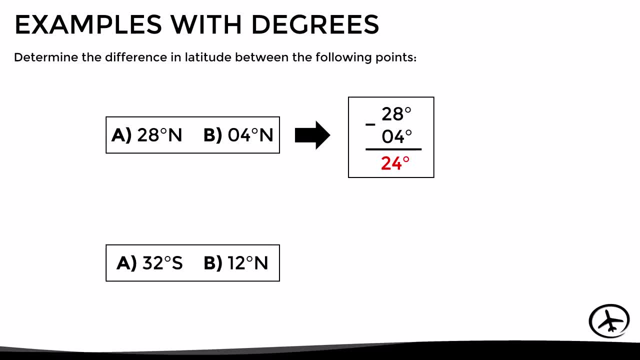 Now, in this second case, the points are in different hemispheres, so we just add the latitudes to obtain a difference in latitude of 44 degrees. Now, up to this point we have only used degrees for the examples. Let's see how to do this operation with degrees in minutes. 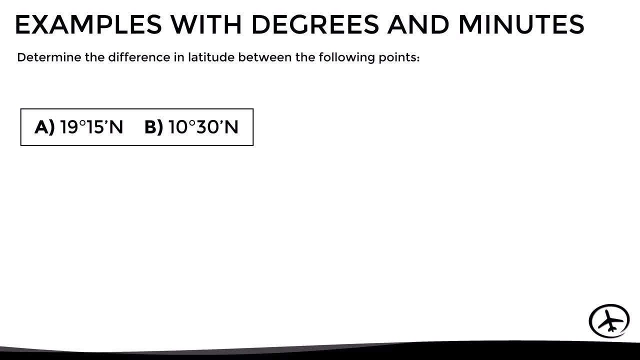 In this first case, since both points are in the same hemisphere, we just have to subtract the latitudes. However, subtracting 15 minus 30 can be difficult If done manually, so it is better to convert one of the degrees into minutes so that we 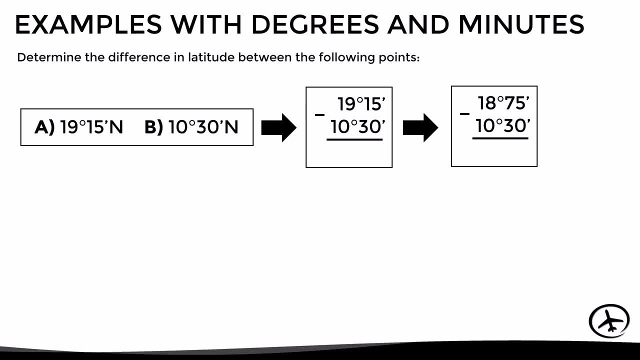 now have 18 degrees in 75 minutes instead of 19 degrees in 15 minutes. This way, the operation is much easier now, and we obtain a difference in latitude of 8 degrees in 45 minutes. Now, in this second case, the points are located in different hemispheres, so we have to add: 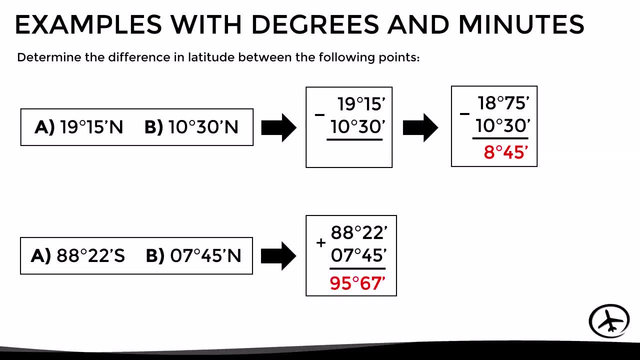 the latitudes. In this case, we obtain 95 degrees in 67 minutes. Now, in this second case, the points are located in different hemispheres, so we have to add the latitudes. In this second case, the points are located in different hemispheres, so we have to add 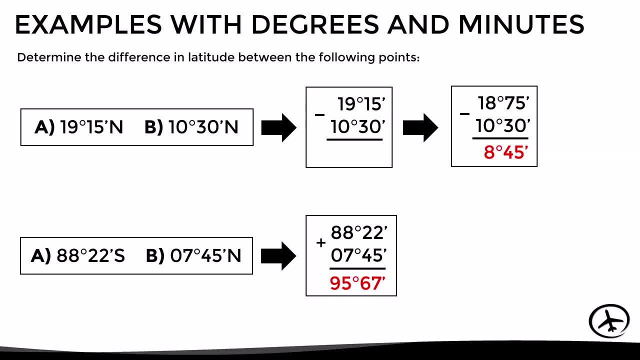 the latitudes. However, to express it correctly, we need to convert 60 of those minutes to 1 degree, then obtaining a difference in latitude of 96 degrees in 7 minutes. Now, having seen the difference in latitude, let's now look at the difference in longitude. 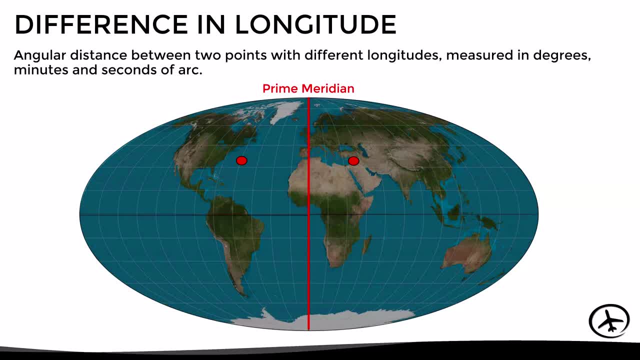 The difference in longitude is defined as the angular distance between two points with different longitudes, measured in degrees, minutes and seconds. So it is basically the same as the difference in longitude. So it is basically the same as the difference in longitude, But now in terms of longitude. 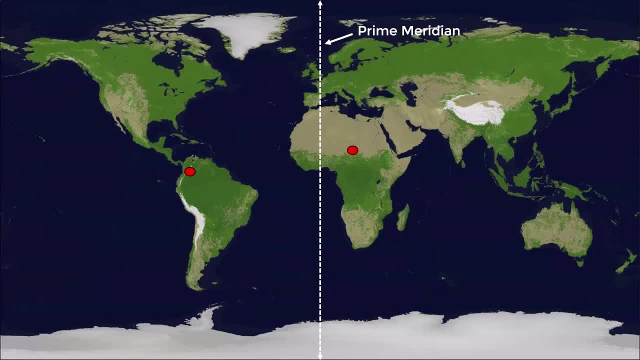 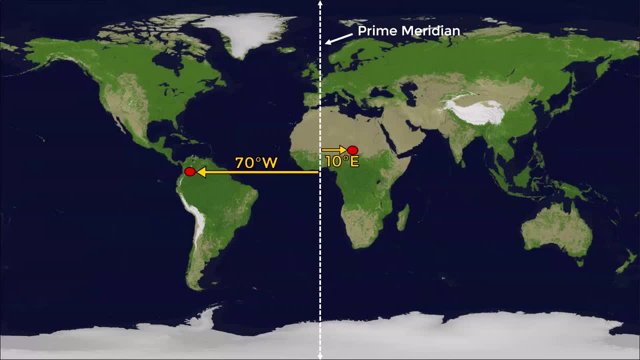 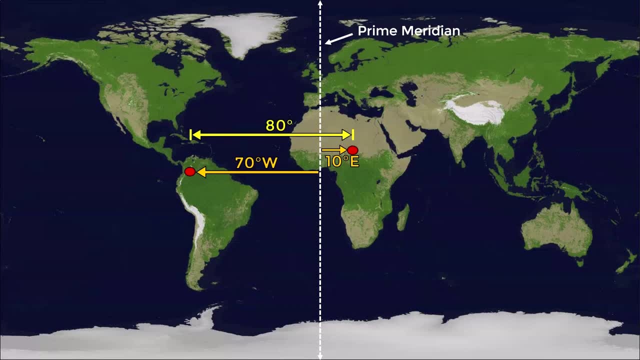 Here the difference in longitude would be 80 degrees. Here the difference in longitude would be 80 degrees. And in this other case, where the longitudes of the points are 90 degrees east and 50 degrees east, the difference in longitude would be 40 degrees. 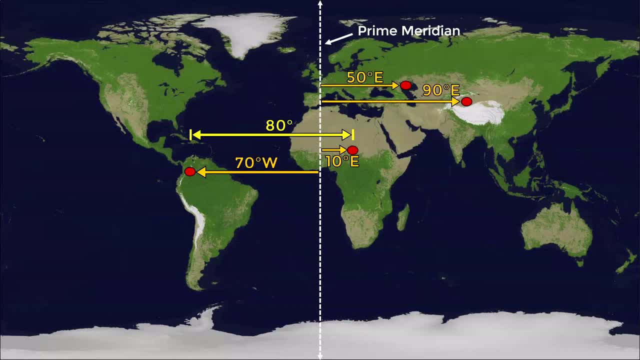 And in this other case, where the longitudes of the points are 90°E and 50°E, the difference in longitude would be 40°. As, with latitude to obtain the difference in longitude, these must be added or subtracted. 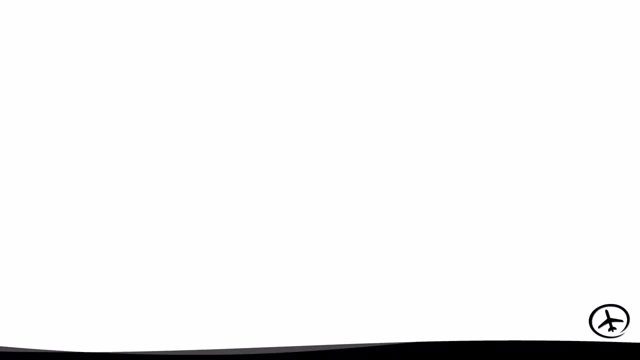 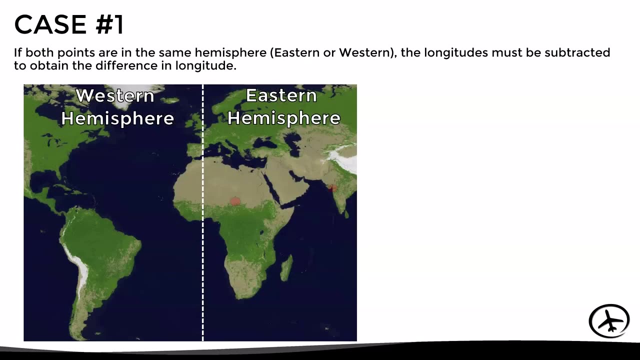 depending on the case. If both points are in the same hemisphere, then the longitudes must be subtracted to obtain the difference in longitude. So in this example, since both points are in the eastern hemisphere, then we subtract the longitudes and obtain a difference in longitude of 60°. 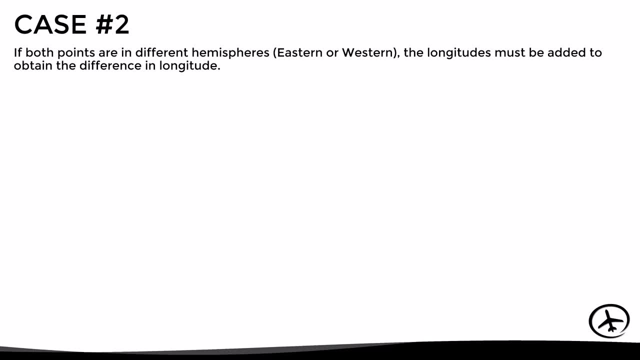 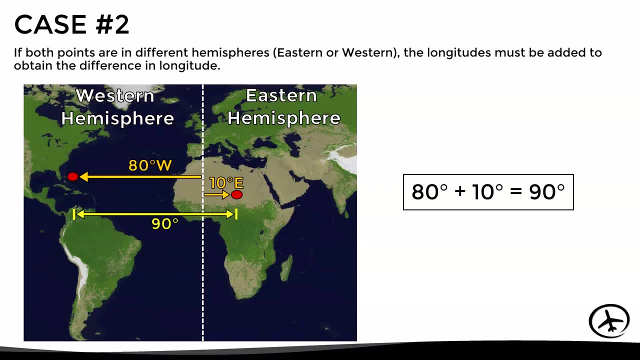 On the other hand, if both points are in different hemispheres, the longitudes must be added. So in this case we just add the longitudes and obtain a difference in longitude of 90°. Let's now look at some examples using degrees and minutes. 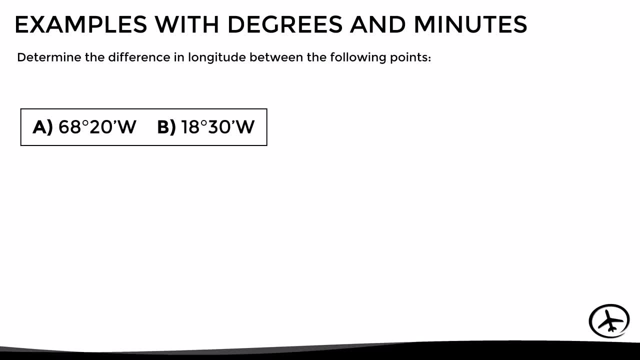 In this first case, both points are in the western hemisphere, So we have to subtract the longitudes. However, as we have already seen, subtracting 20 minus 30 can be difficult if done manually, So it is better to convert one of the degrees into 60 minutes, so that we now have 67° and 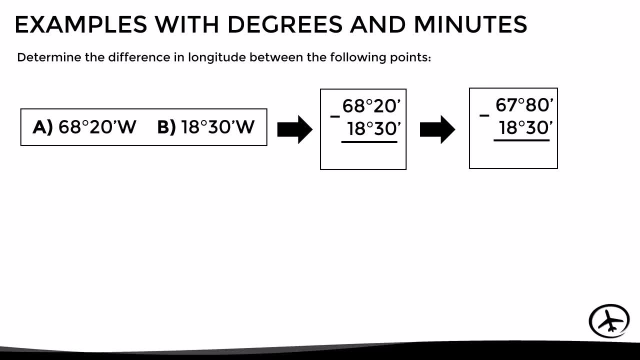 80 minutes instead of 68° and 20 minutes. This way, the operation is much easier and we obtain a difference in longitude of 49° and 50 minutes. Now, In this other case, the points are located in different hemispheres, so we have to add. 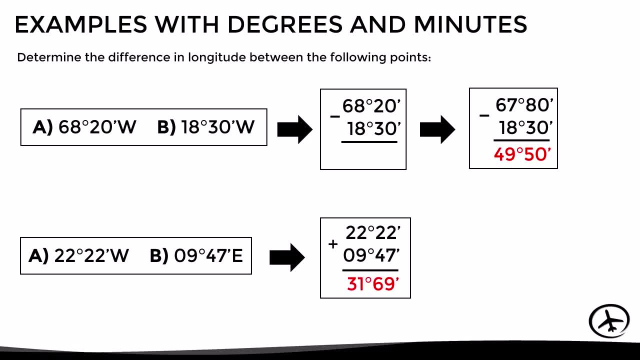 the longitudes. Here we obtain a difference in longitude of 31° and 69 minutes. However, to express it correctly, we must convert 60 of those minutes into 1°, So we get 32° and 9 minutes. So, having seen how to obtain the difference in latitude and longitude, let's look at 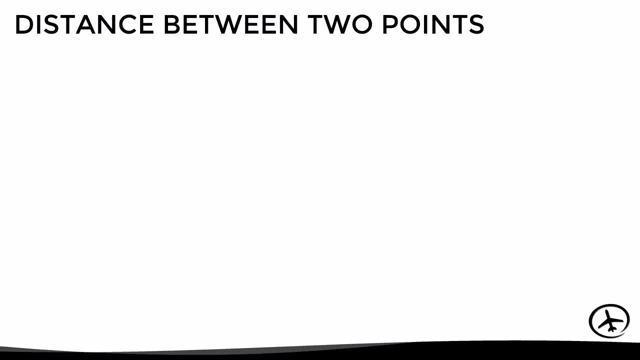 how to convert it into distance. As we previously mentioned, the distance between two points on the Earth's surface can be measured in angular terms, since it is a sphere. However, angular distances are not used for navigation purposes, since other units of linear distance are used, such as nautical miles, kilometers, etc. 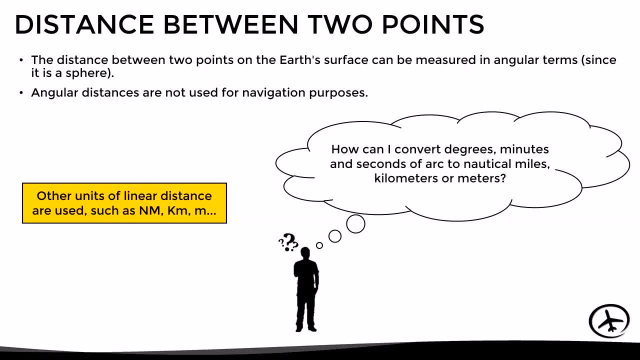 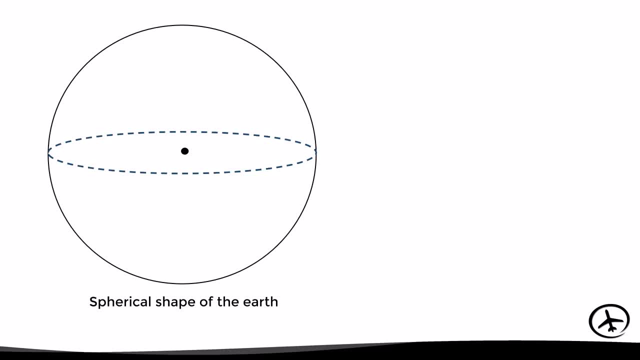 So the question is: how can we convert degrees, minutes and seconds of arc to nautical miles, kilometers or meters? Well, To answer this, We must first analyze the dimensions of the Earth. In practical terms, we can assume that the Earth is a perfect sphere with a circumference. 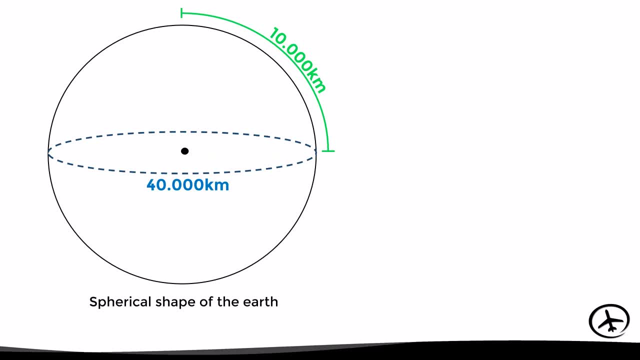 of 40,000 kilometers. With this in mind, we can then say that if 360° equals 40,000 kilometers, then each degree equals 111.11 kilometers And, as we know, each degree can be divided into 60 minutes. 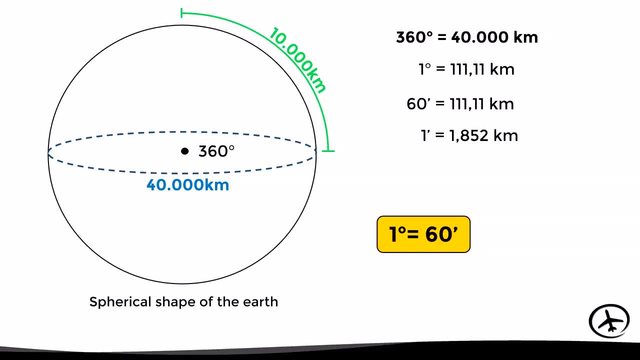 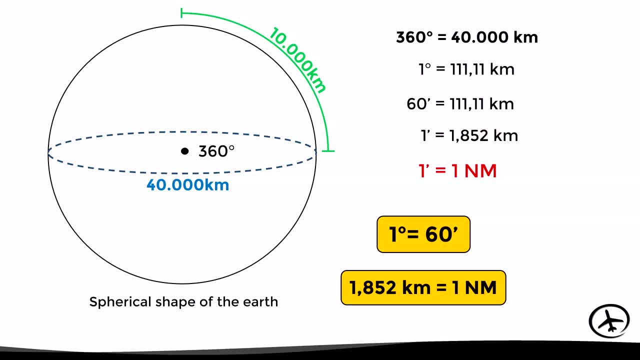 So then we can say that each minute of arc equals 1 nautical mile. However, as we will see later, this rule is not true in all cases. In fact, this rule only applies when both points are on the equator or on the same meridian. 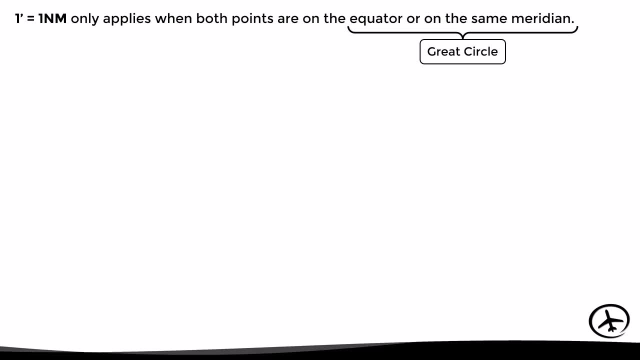 which are great circles. But let's see why. At the equator, the circumference of the Earth is 40,000 kilometers, As we said before, which means that here each minute of arc equals 1 nautical mile. However, if we move towards the poles, for example at 60° of latitude north or south, 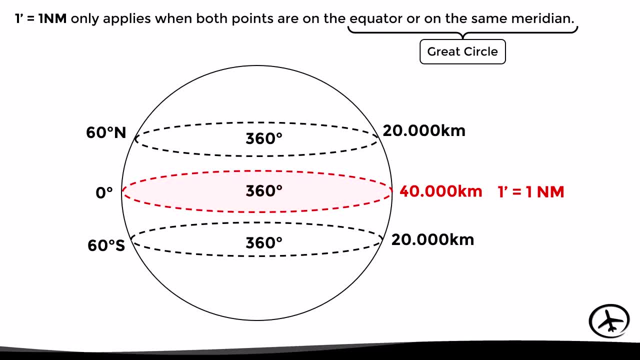 the circumference of the Earth at this point is only 20,000 kilometers, which means that here each minute of arc equals 0.5 nautical miles, And if we move further towards the poles, we will see that the circumference becomes smaller and smaller. 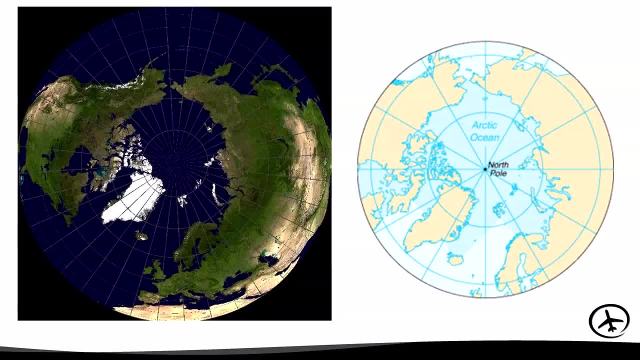 This can be seen more clearly if we look at the Earth from one of its poles. As we can see here, the circumference of the parallels gets smaller and smaller as we approach the pole, so that the same angular distance in terms of degrees and minutes will be equivalent. 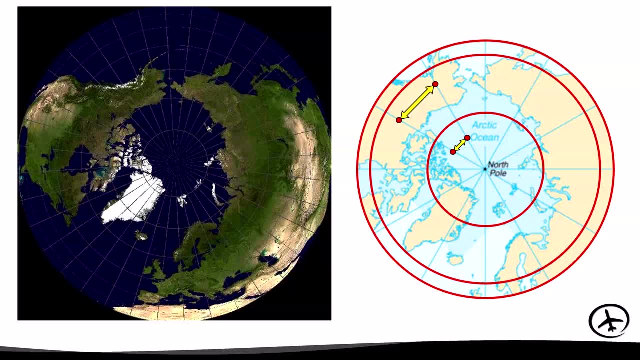 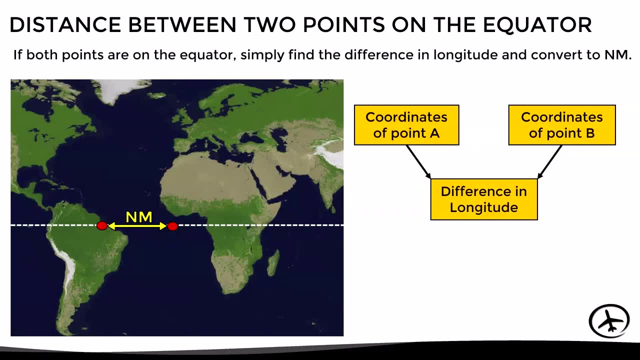 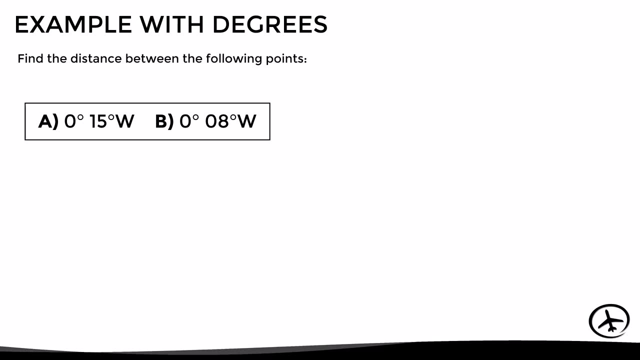 to a smaller linear distance in terms of nautical miles. In this order of ideas, if both points are on the equator, we just have to find the difference in longitude and convert it to nautical miles. Let's see an example Here. the latitude of both points is 0°, which means that they are both on the equator. 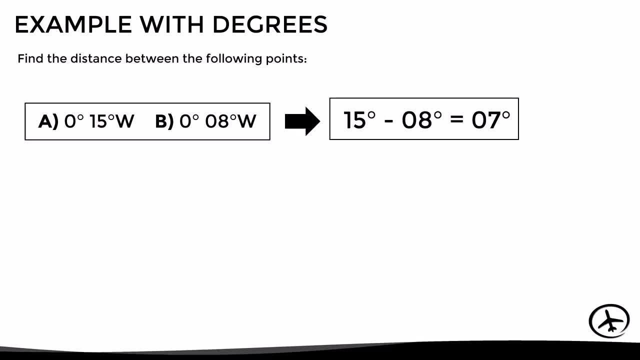 So, to determine the difference in longitude, we just have to subtract the longitudes, obtaining 7° as a result. Now, since each degree equals to 60 minutes, this means that the difference in longitude can be expressed as 420 minutes. And since, at the equator, each minute equals 1 nautical mile, this means that the linear 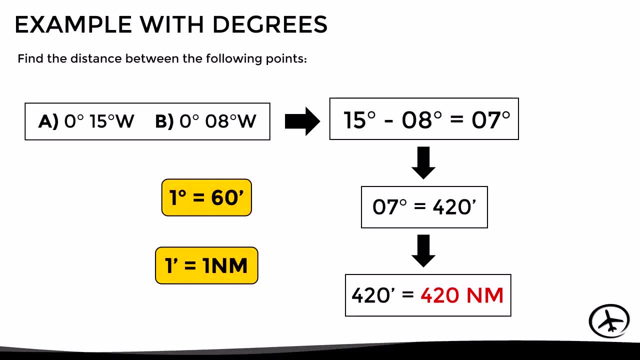 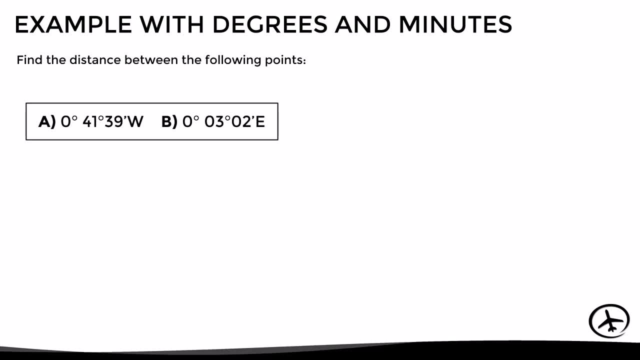 distance between these two points is 0.5 nautical miles. Now let's see another example, but now with degrees and minutes. In this case, these points are both at the equator and since they are in different hemispheres, we have to add the longitudes to obtain the difference in longitude, which, in this case, 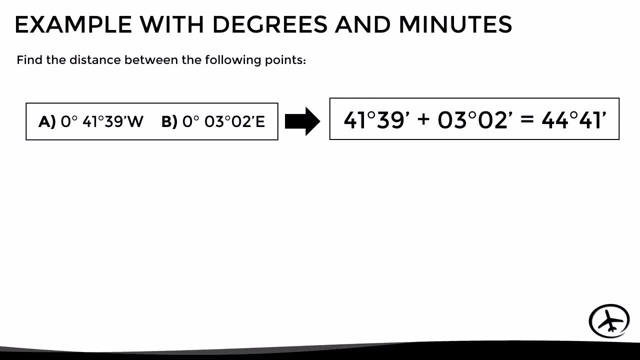 is 44° and 41 minutes. Now, since each degree equals to 60 minutes. if we convert 44° to minutes, the result will be 2640 minutes plus the remaining 41 minutes. This way, since each minute equals 1 nautical mile at the equator, the distance between 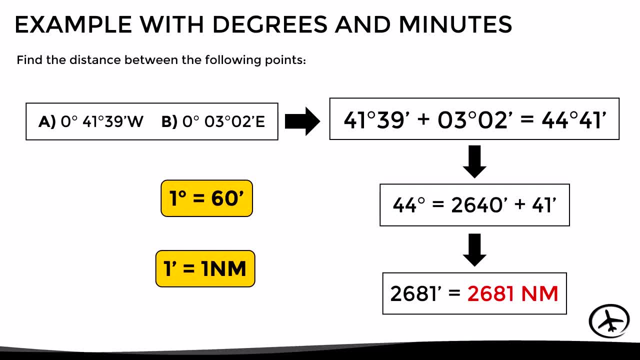 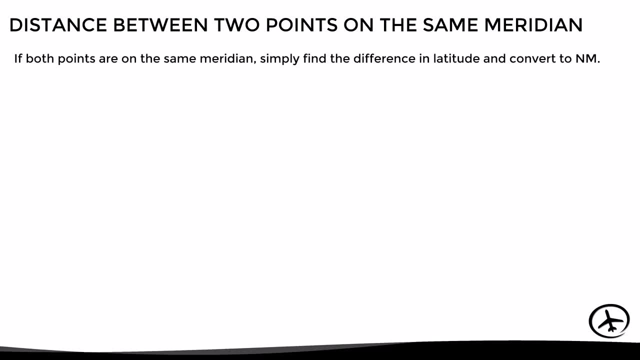 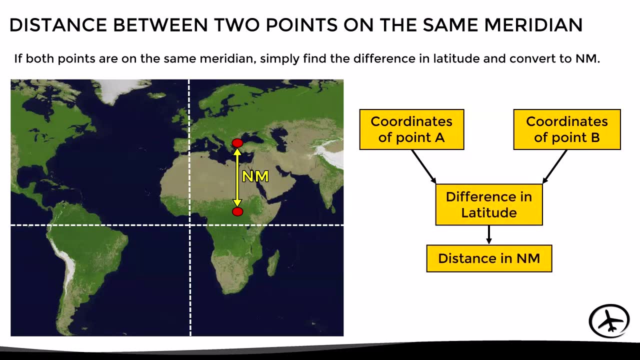 both points is 2681 nautical miles. Now a similar procedure applies when both points are located on the same meridian. In this case, we just have to determine the difference in latitude and then convert it to nautical miles. Let's see an example. 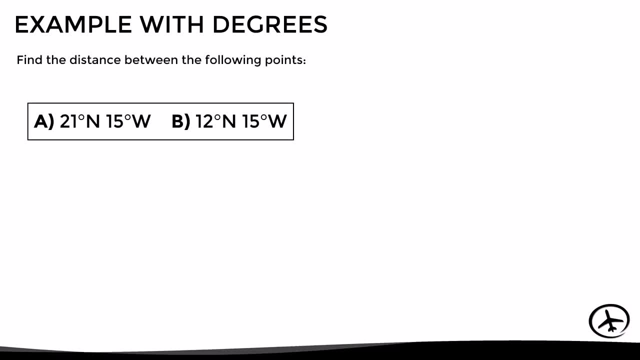 Here. as we can see, both points are on the same meridian, which is 15° west. So to determine the difference in latitude, we just have to subtract the latitudes, obtaining 9° as a result. Now, if we convert 9° to minutes, the result will be 540 minutes. 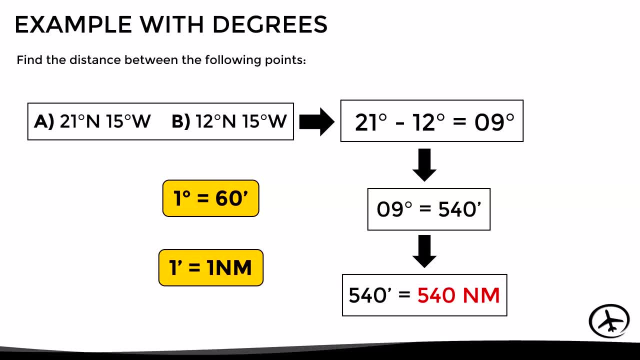 And since, on the same meridian, 1 minute equals 1 nautical mile, this means that the distance between these points is 540 nautical miles. Now let's see another example Here. as we can see, both points are on the same meridian, which is 15° west. 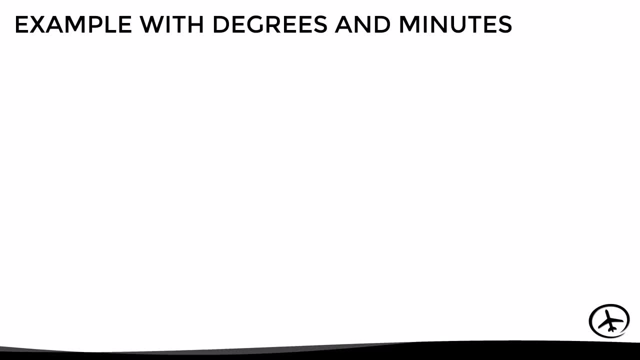 So to determine the difference in latitude, we just have to subtract the latitudes obtaining 9° as a result. So to determine the difference in latitude, we just have to subtract the latitudes obtaining 9° as a result. And since, on the same meridian, 1 minute equals 1 nautical mile, this means that the distance 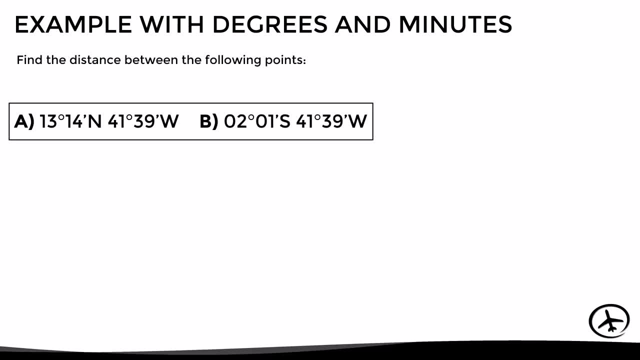 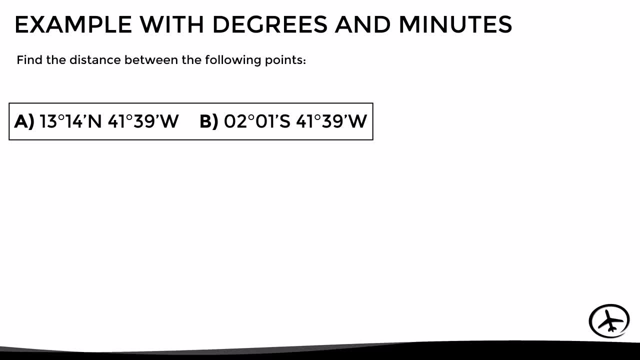 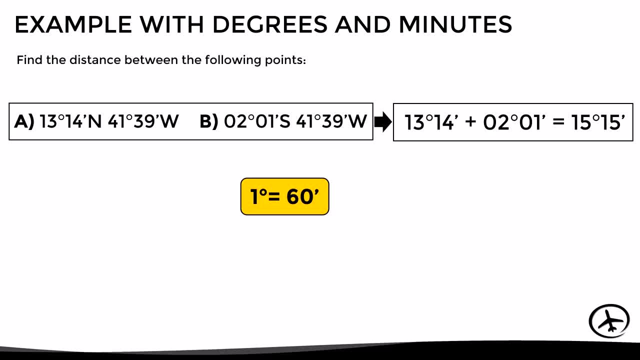 degrees in 15 minutes. This way, if we convert 15 degrees to minutes, we obtain 900 minutes plus the remaining 15 minutes, which means that the distance between both points is 915 nautical miles. Now, so far we have seen the simplest cases where the rule of 1 minute equals 1 nautical mile can be. 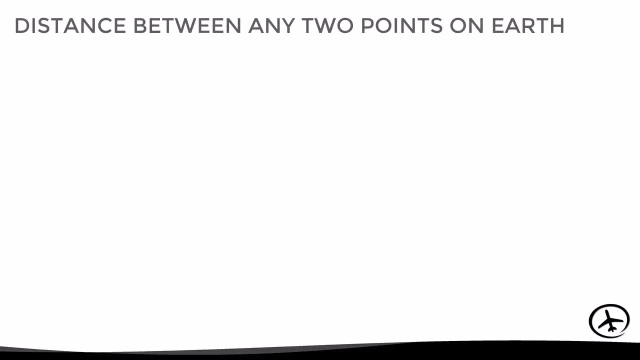 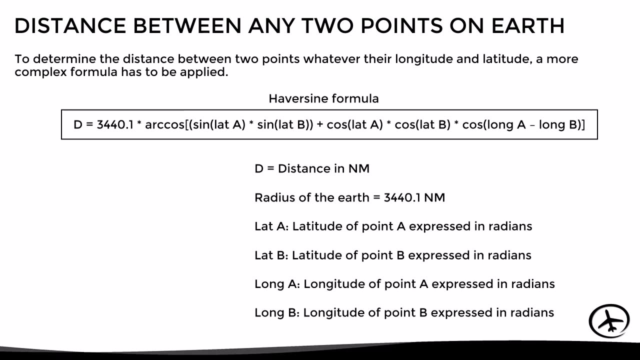 applied. However, if what we want is to calculate the distance between two points independently of their latitude or longitude, we can do it by means of a more complex formula known as the Haversine formula, which is this one. What this formula does is to create a fictitious great circle. 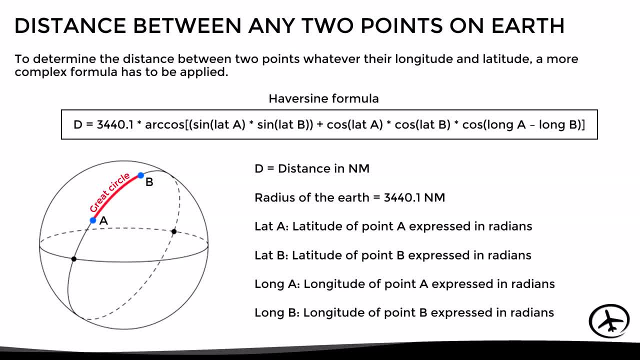 that passes through the two points. we are interested in allowing us to determine the shortest distance between those points. One important thing to bear in mind is that the latitudes and longitudes of the two points are the same, So if we want to calculate the distance, 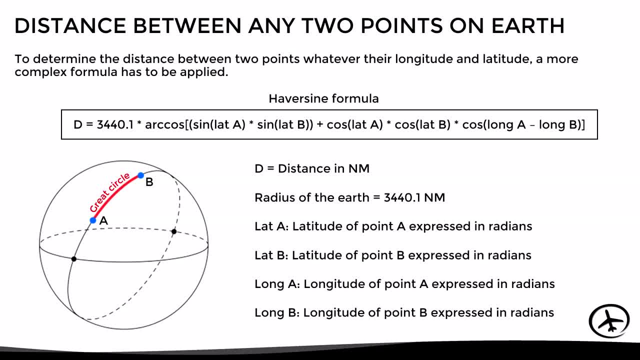 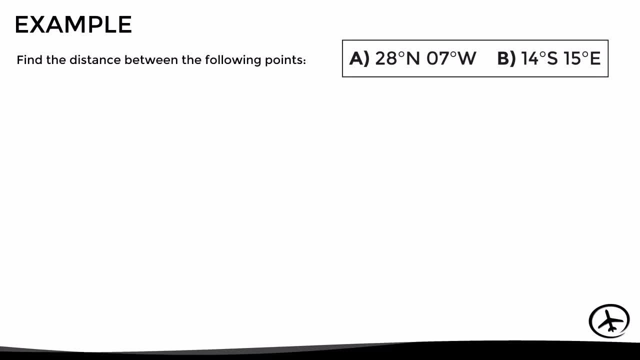 between two points, independently of their latitude or longitude. we must convert them to radians to introduce them in the formula. Let's see an example of how to use it. Suppose we want to determine the distance between these points. so here we have the corresponding latitudes and 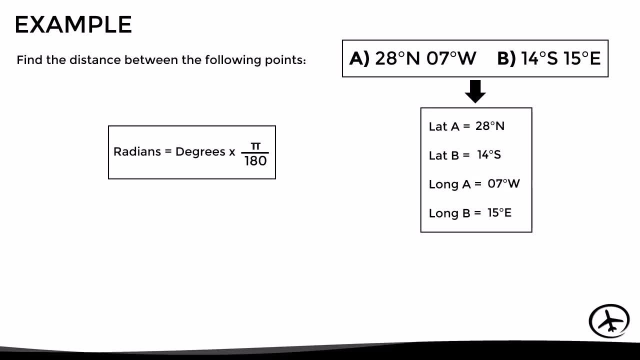 longitudes. However, in order to convert them to radians, it is necessary to change the sign according to the hemisphere. In this case, the northern and eastern hemispheres are positive, while the southern and western are negative. After doing this, we can now convert them to radians using this formula. Once this is done, we can now replace: 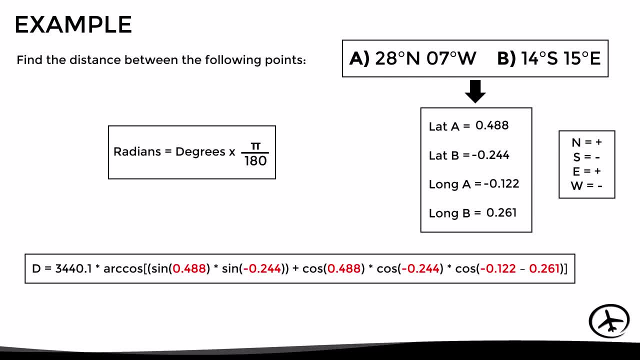 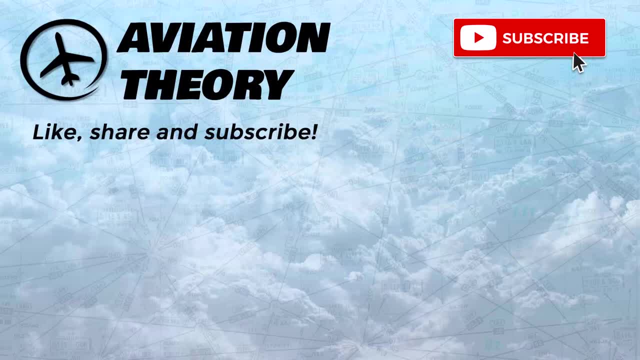 them in the formula and do the math, obtaining as a result a distance of 2827.7 nautical miles. I hope the information presented in this video was useful. If so, don't forget to share, like, subscribe and leave a comment down below. Thanks for watching.